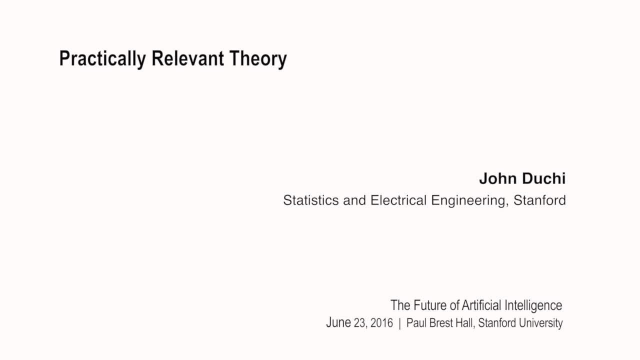 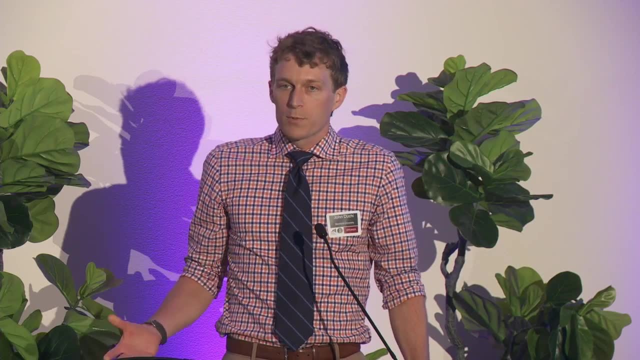 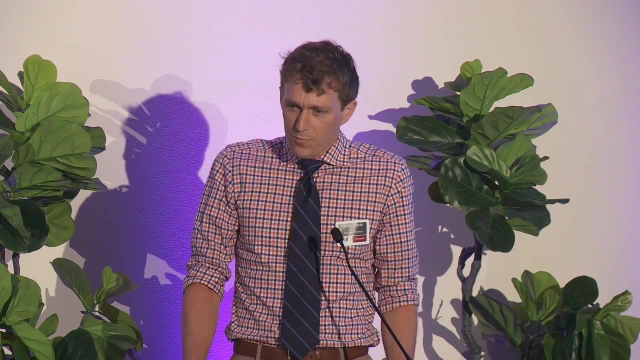 Hi everyone, Thanks for the opportunity to speak to you. So I'm going to try to talk about some of the work that my group has been doing on kind of building connections between theoretical research and practical relevance. So let me just start by enumerating a number. 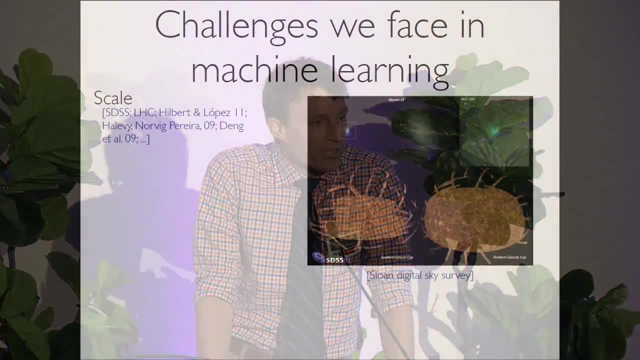 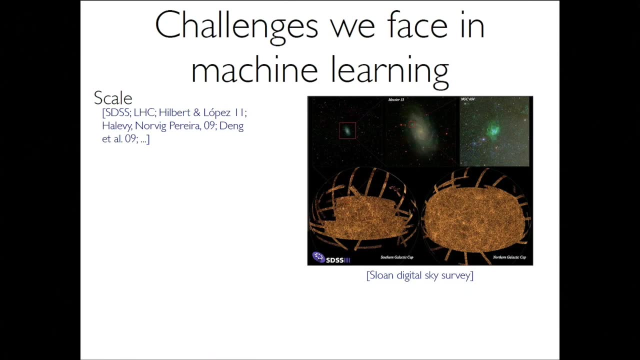 of the challenges we face in machine learning Scale. a huge challenge, right. The Sloan Digital Sky Survey, in the first month of its existence, had collected more data than the sum of all previous astronomical experiments. Well, Fei-Fei's group, as you saw, has been. 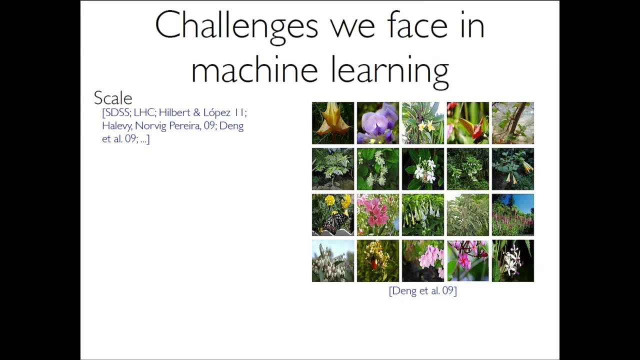 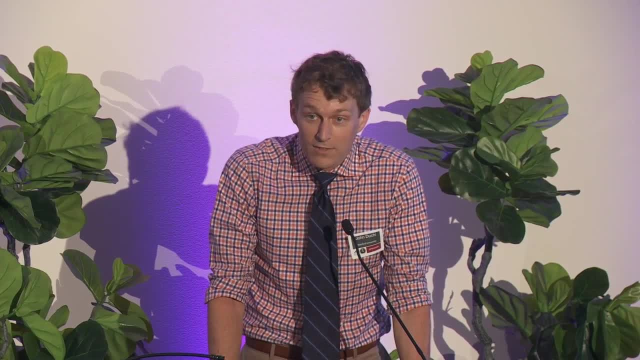 generating these gigantic image data sets. I mean, how many gigabytes do you guys have now in ImageNet? How big is ImageNet now? Fifteen million images, right, So that's big. We're getting all sorts of types of data, you know, social network data, things like. 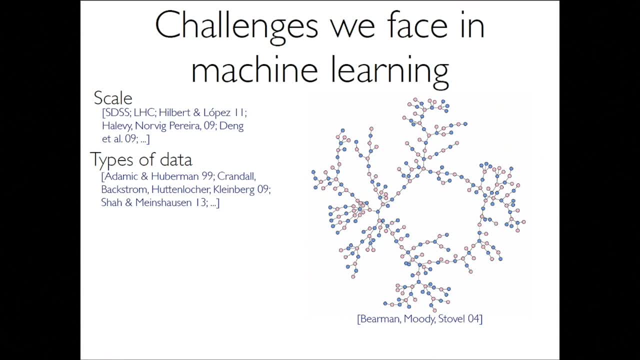 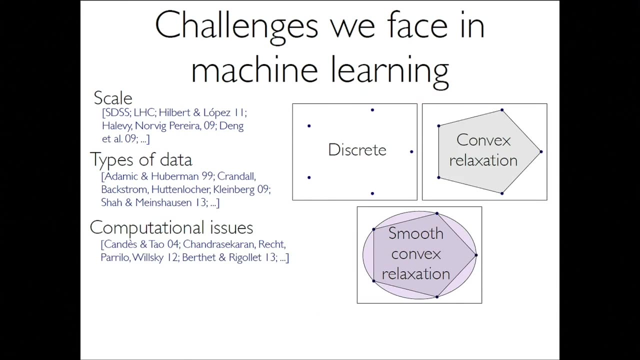 that. that are a little bit unusual. This is a dating network from a high school. I wish I had a laser pointer, because there's some really good nodes in the network, but I don't have a laser pointer, so you guys will have to come back and look for that. 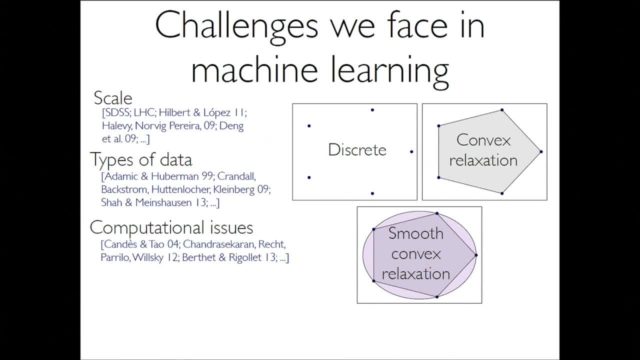 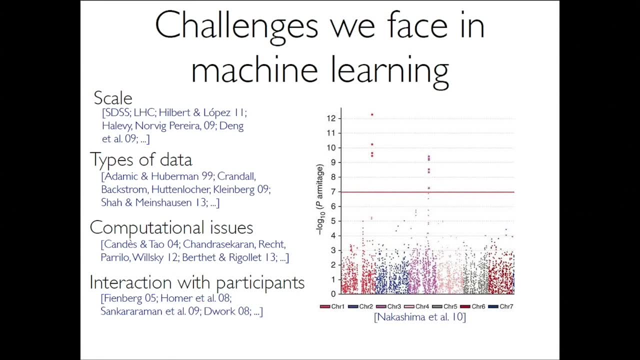 We face computational issues. you know computational hardness. We want to compute things very efficiently. You know, as we collect more data, the sort of interaction that our algorithms kind of force upon participants. you know privacy compromises- things like that start to come. 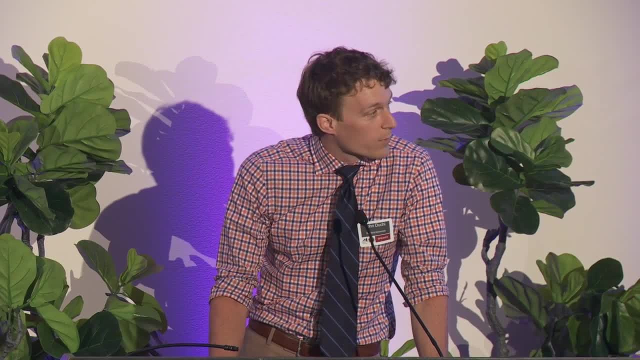 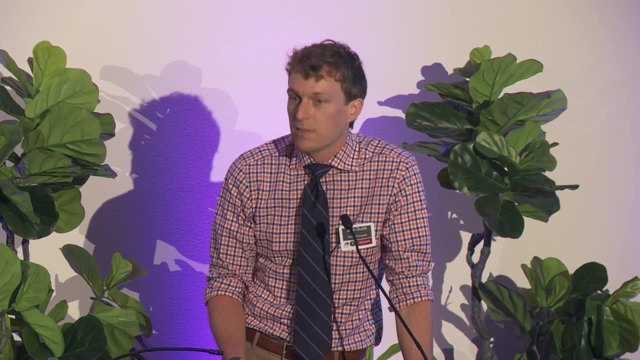 up right. So in 2008, some- Richard, Nils, Homer and some colleagues showed that you know, just by using count data in genomics, you could actually figure out who belonged to different medical studies. This caused the NIH to stop releasing data for a while, and 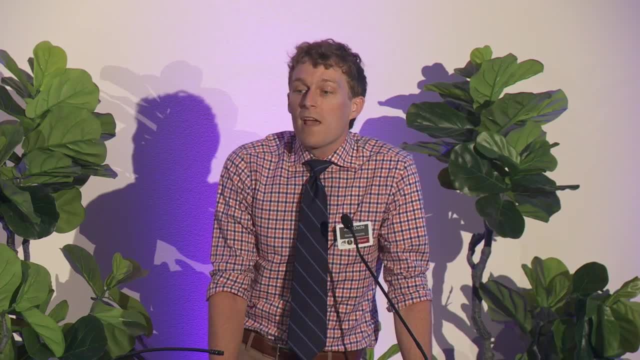 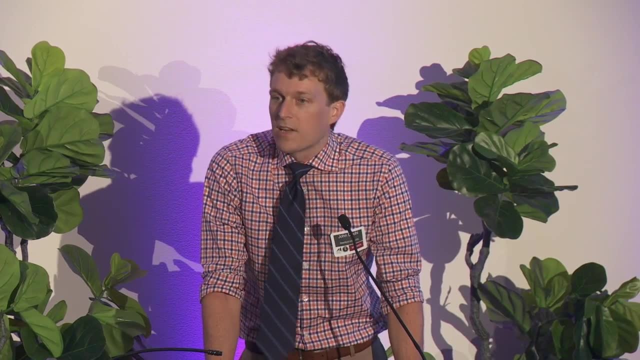 that's kind of a problem, right, We need data from the NIH to be able to do things, And so what I try to do is—there we go—incorporate these kinds of issues into sort of analyses of machine learning algorithms and develop procedures that kind of automatically trade. 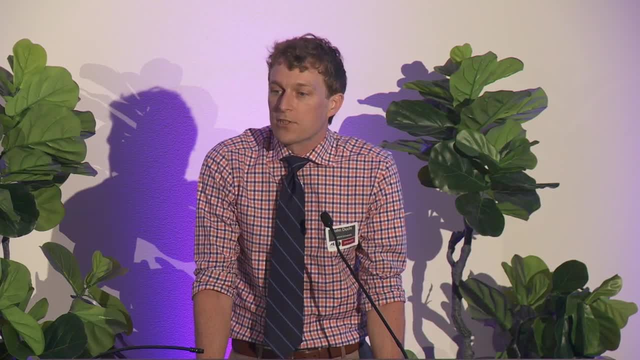 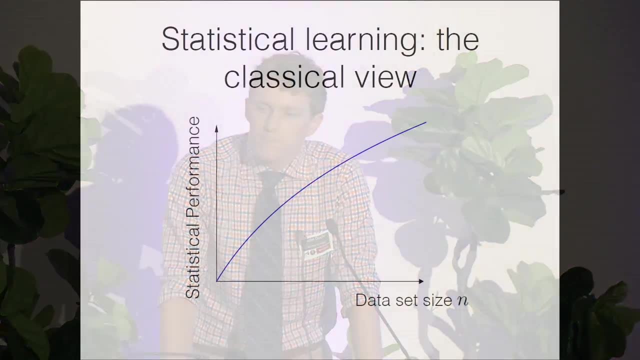 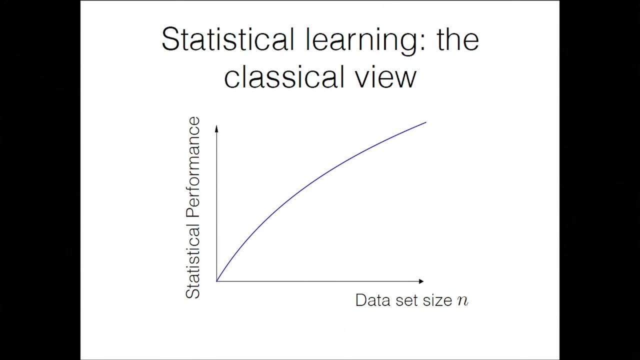 off between these different types of difficulties and challenges. So the kind of classical view in statistics and machine learning is that we get more data and we get better performance. right, There's kind of two axes: Data set, size grows, performance gets better. And I think this is the wrong view to take. now We need to actually have 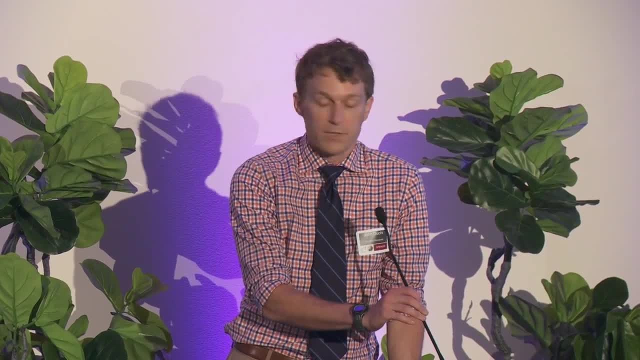 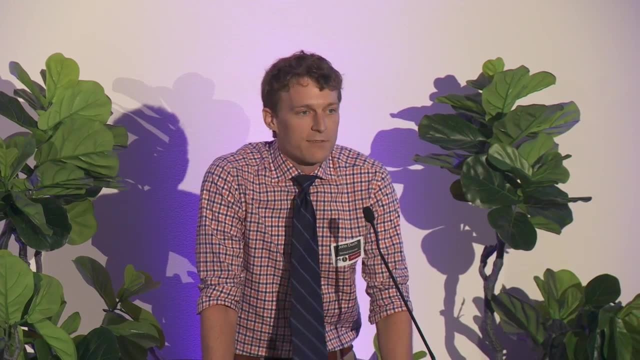 a much kind of broader view, either as theoreticians or as practical people. You know, it's not just how much data we've collected, There are additional things we have right. So we want kind of these 3D or more pictures where we say, okay, we have, you know, we have a. 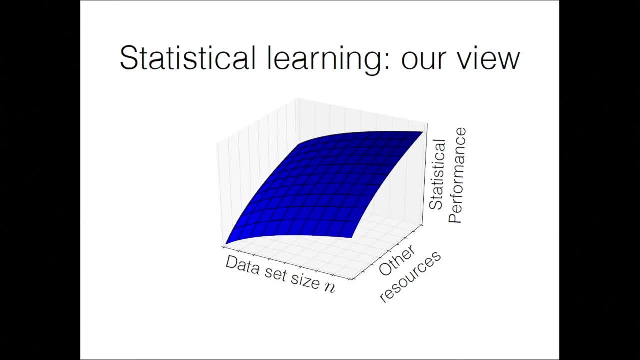 multiple axes along which we want to measure performance. We want to have you know the amount of data we need to collect. We have you know our statistical performance, how good the inferences we make are. And then there's some other resource constraints or 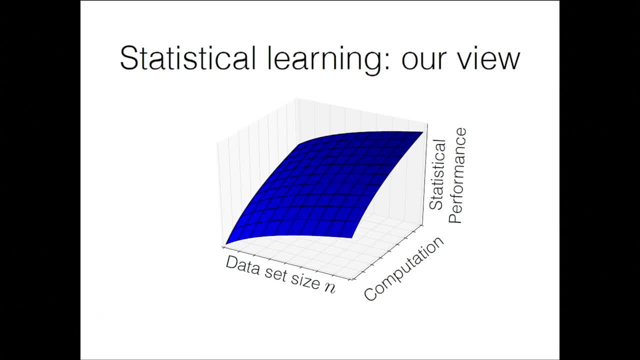 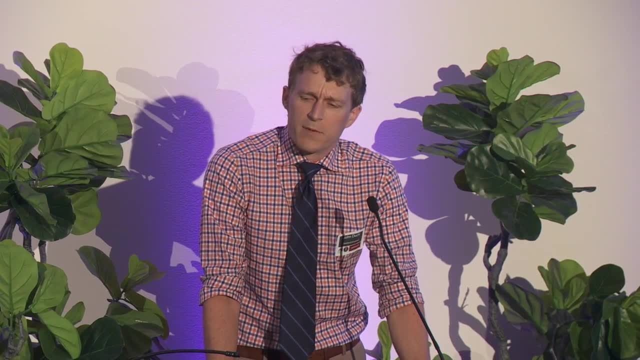 considerations that we want to take into account. This might be: you know how much computation is it going to cost? How many icebergs are we melting by computing these things right? I guess energy use does the same thing We might care about. you know how many sort 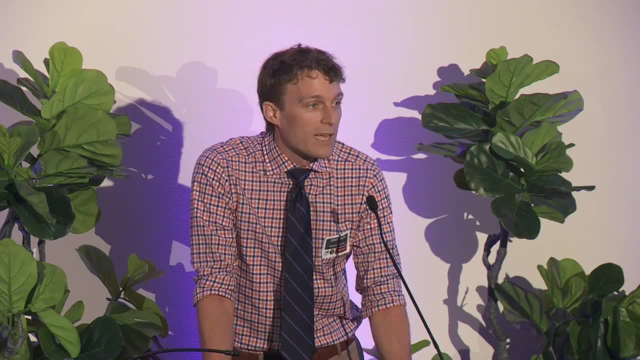 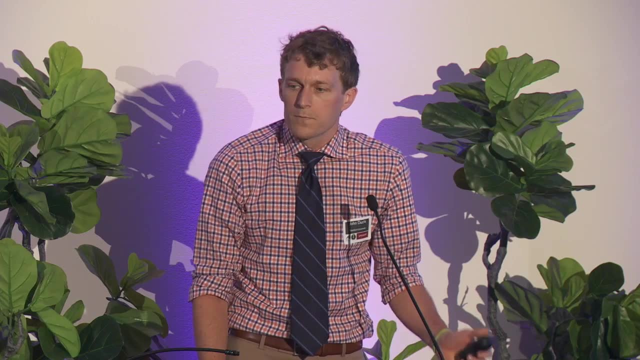 of sensitive disclosures does our—do our machine learning algorithms—do our machine learning algorithms make? Or how much sort of sensitive data do we need to collect to actually do things And so—whoops. So my research, you know, tries to make connections. 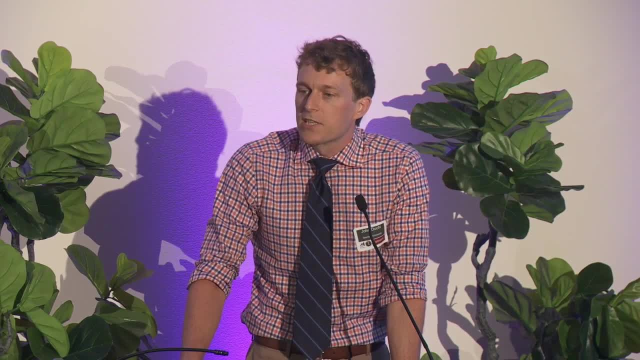 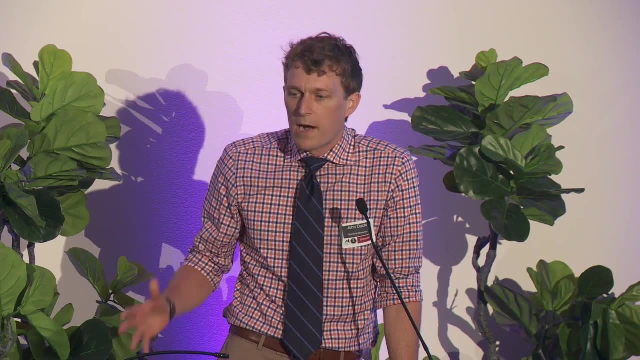 between machine learning, optimization, information theory and statistics, and we try to take this sort of two-part view where we try to develop algorithms that kind of optimally do things, basically improve performance. So we want to, you know, push the performance. 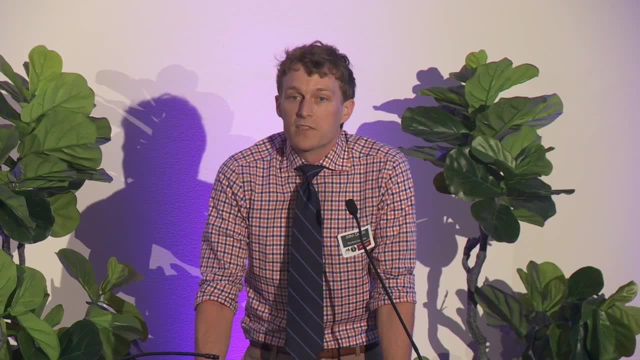 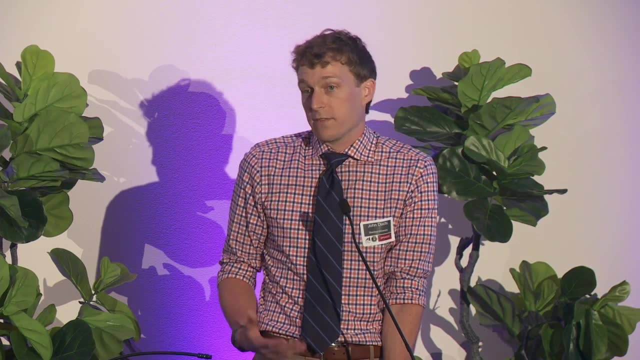 up as high as we can. but we also want to understand fundamental limits So we can say: hey look, you know, I've come up with a procedure and it's provably optimal. You know, and these—understanding what these limits are- will allow us to kind of on the 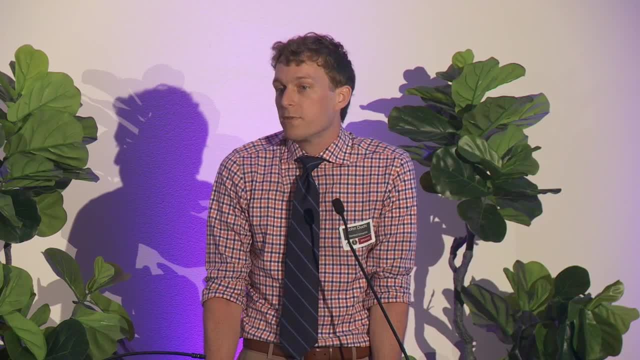 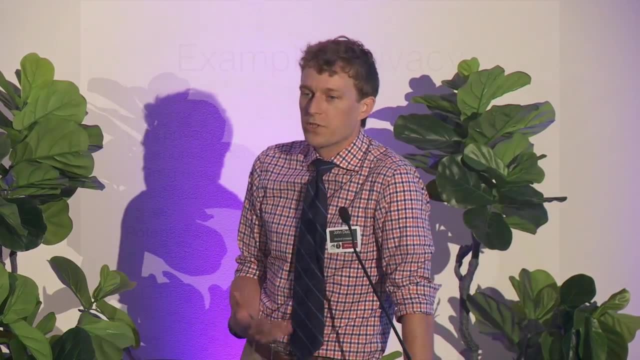 flip side, develop better procedures or know when it might be possible to develop a better procedure, So let me you know—so there's a number of examples where this can happen, but let me dig into one which is some of my work in privacy. So why privacy right? 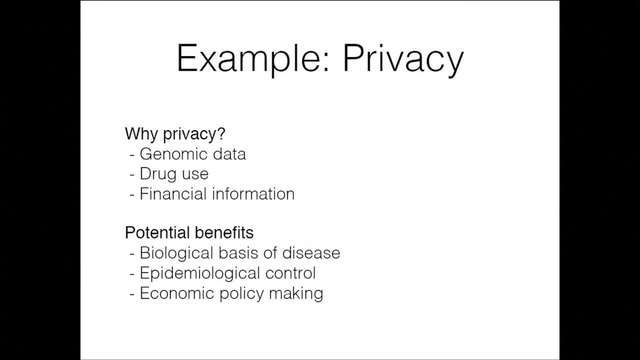 There are many situations where we have data that you might want to keep private. You know your genomic data- whether you use drugs, things like this, your financial status. you know financial information. Of course, there are many potential benefits, both policy and 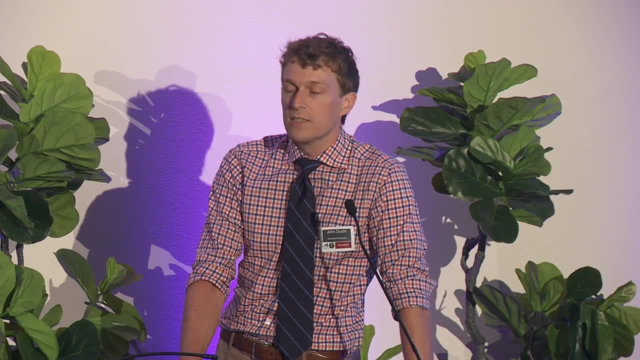 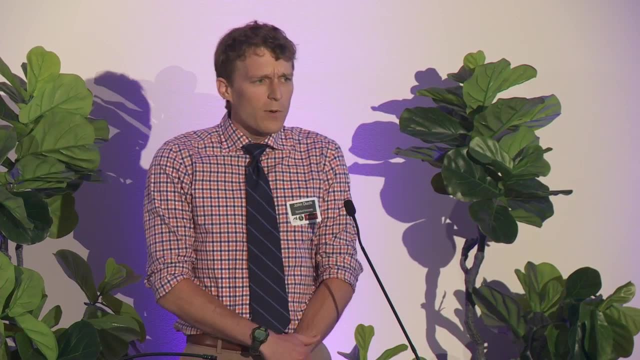 science-wise, You know, we might want to understand better biological bases of disease, do better epidemiological control or make better economic policies, All right. And so the big question here is: what are the fundamental tradeoffs between, say, privacy and statistical utility? 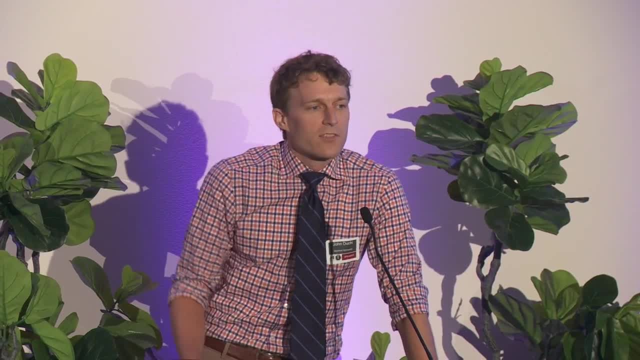 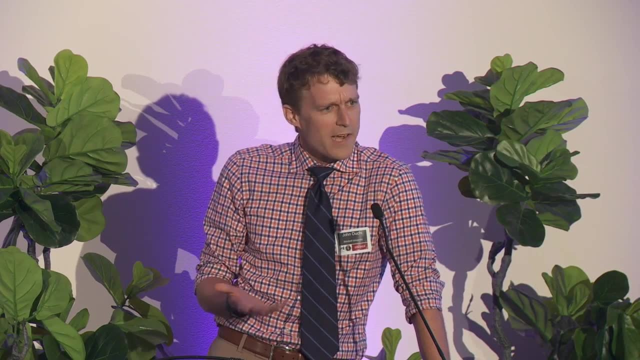 Now let me start with a once provocative question. So I think this is no longer provocative after your boss—I think his quote was: you know, of course, inhalation was the point, something like this: Is that right, Yeah? So this is not. 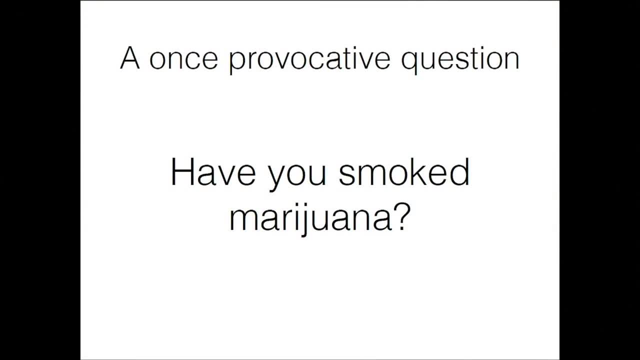 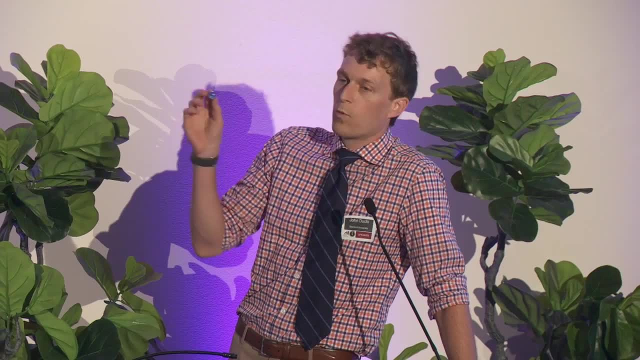 as provocative as it once was, but I'm going to demonstrate a privacy-preserving procedure, So I'm going to roll this die and if it comes up one or two, I'm going to lie when I answer this question to you guys. And if it comes up three, four, five or six, I will tell. 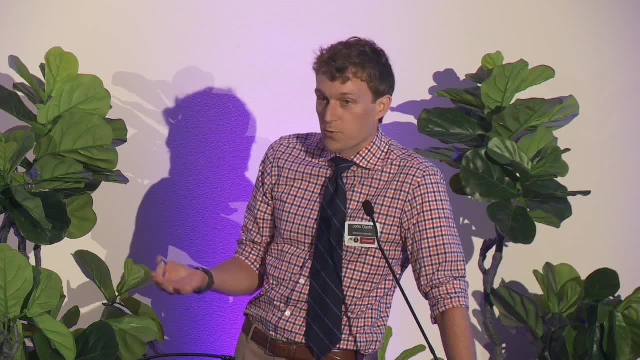 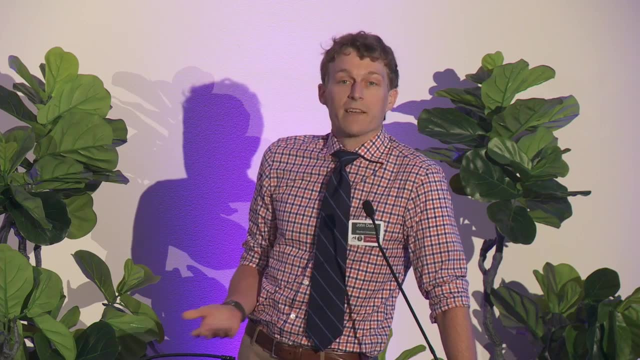 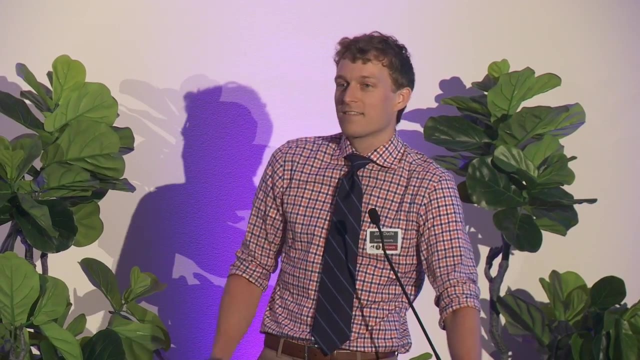 the truth, right. So with probability two-thirds I'm telling the truth. With probability one-third I'm going to lie, but you guys won't know which one I'm doing. All right, So I just rolled the die And I have never smoked marijuana. I haven't right, I mean I haven't at least according. 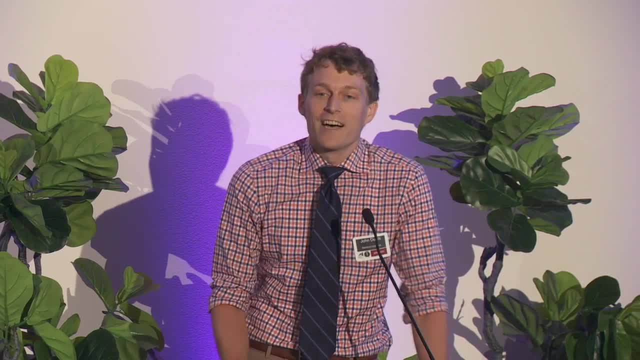 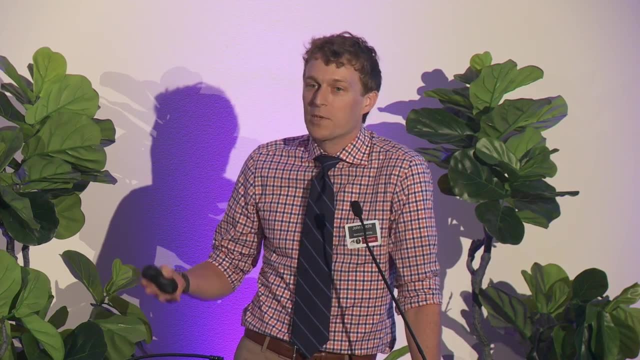 to what the dice said. Okay, Anyway, so that right there actually is an optimal way sort of- at least from sort of the information we get for the statistics we want to compute. that trades off, you know, between preserving my privacy. so you guys don't know whether 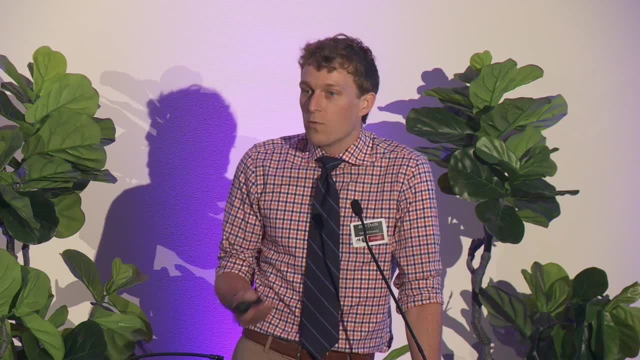 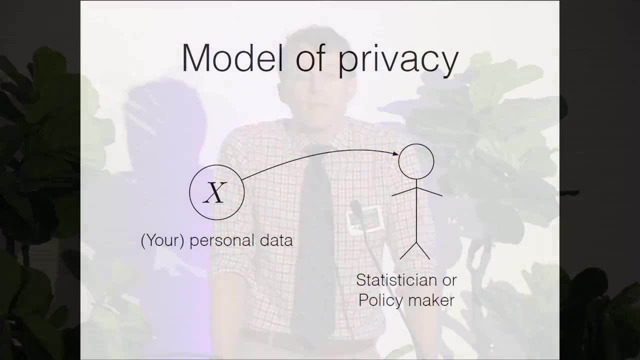 I've actually smoked marijuana and you know what we can actually compute. So to do this, you know. let me just touch a tiny bit on the model of privacy we're going to use. So we have, you know, the classic kind of machine learning, or statistician or 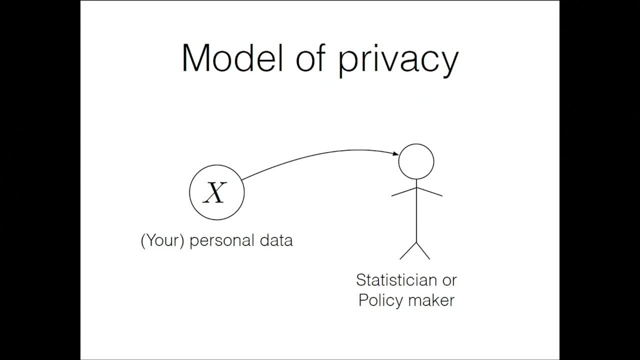 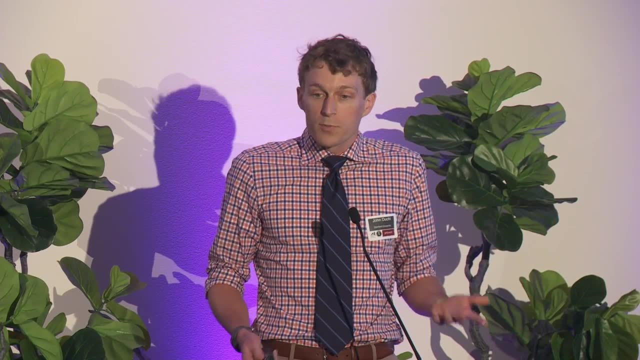 things like that. setting is that there's your data X and then I, the statistician, get to see everything. But you guys don't trust me with good reason, because I do machine learning, statistics, things like this. And so you say: you know what? I want? some protection. 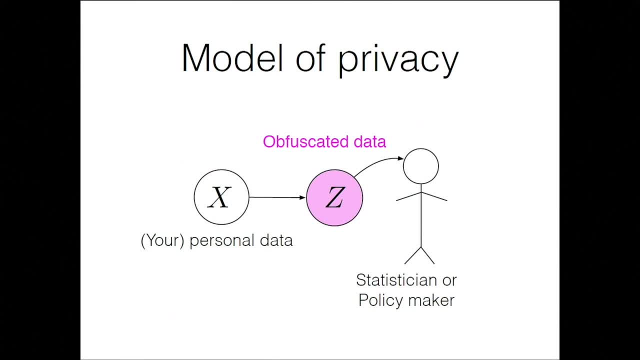 So instead you only let me see some kind of obfuscated data. All right, And formally, what we say is: look, I'm going to give you a guarantee that everything I do is going to be the probability I can distinguish you from some other person, given your obfuscated 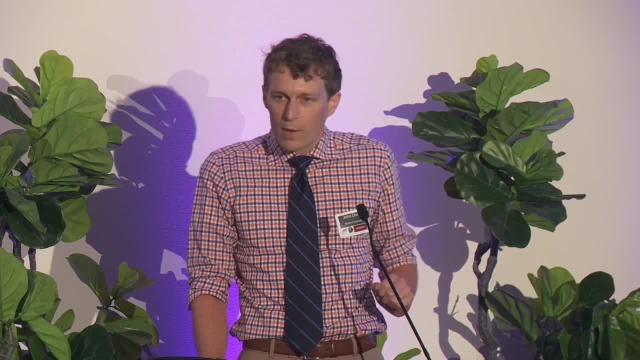 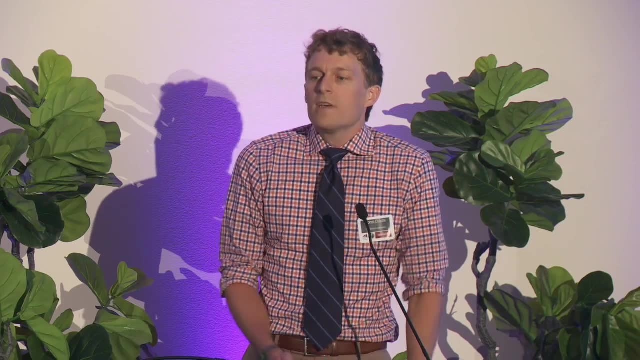 data is less than one half plus a little fudge factor. So I'm almost basically guessing randomly whether the data came from you or not, And I can just do very, very slightly better than random. Okay, And then you know I won't get, and then the goal is: you know.